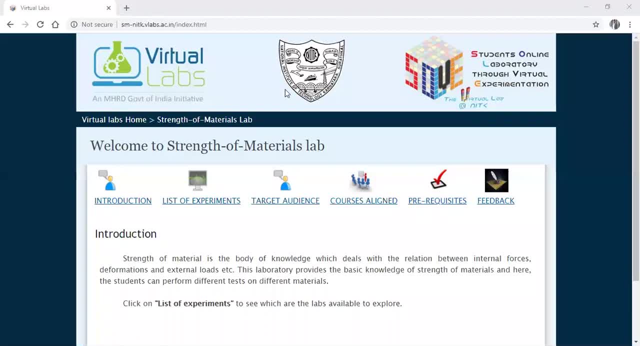 And I also want to thank National Institute of Technology Karnataka, Suratkal, for providing access to all the teachers, students, as well as the researchers to conduct the experiment through virtual labs. Here we are going to see the experiments which are conducted on material testing or strength of material lab. 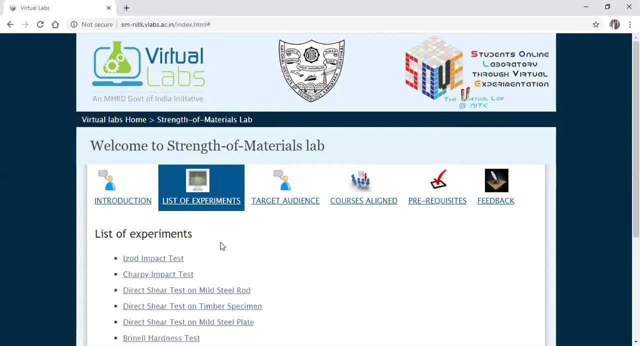 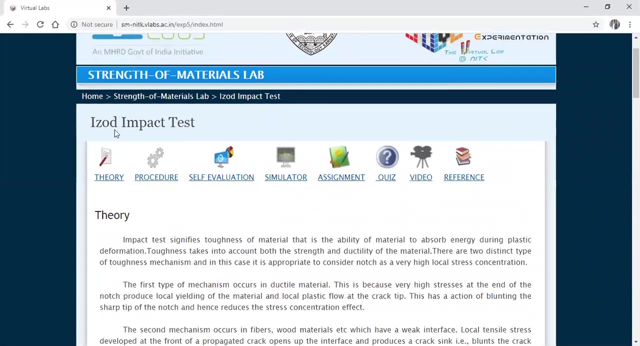 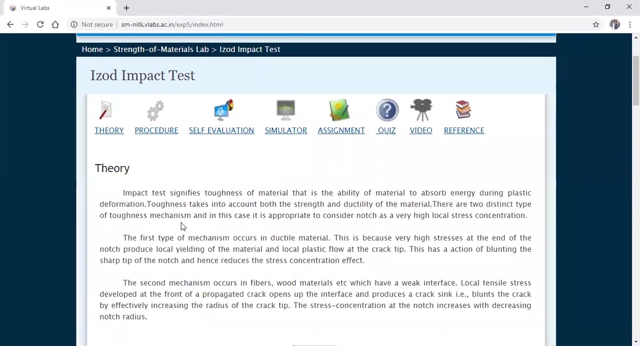 Here are the list of experiments Here. I am interested about the IZOD impact test. Now you can see that the IZOD impact test is open. The first part is the theory they have provided. After that, a procedure is there how you need to conduct the experiment. 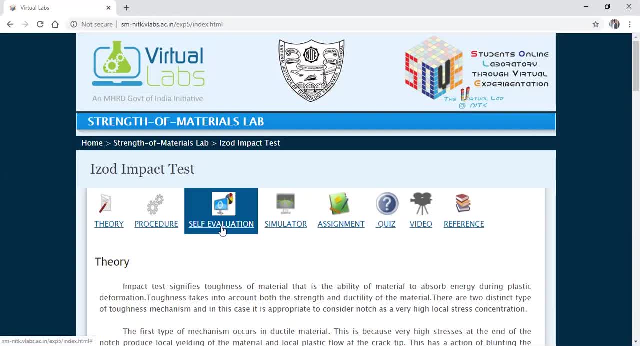 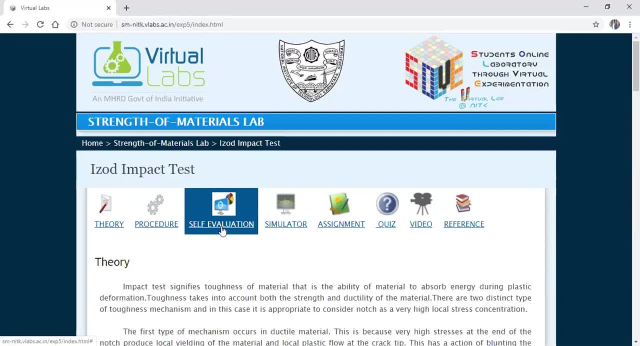 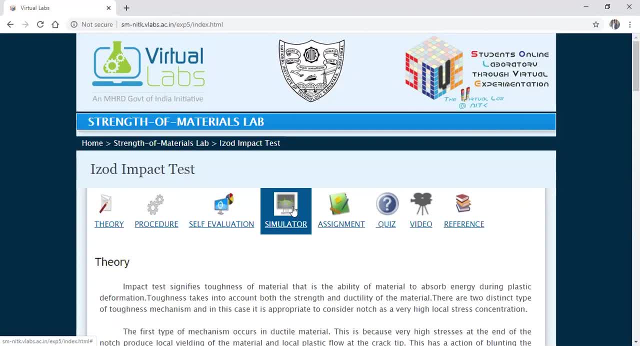 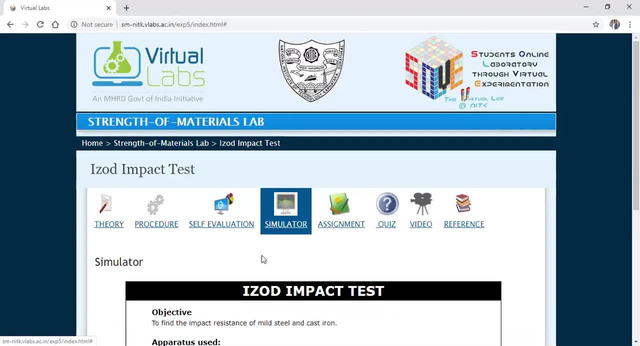 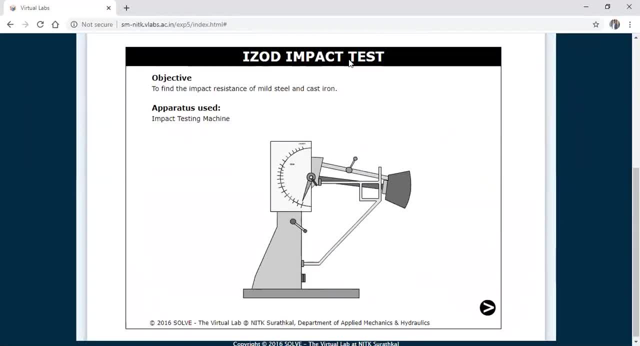 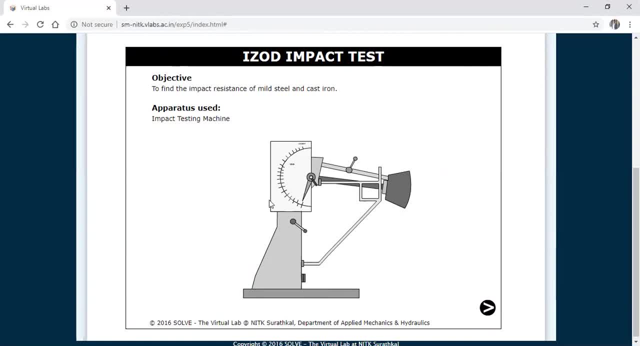 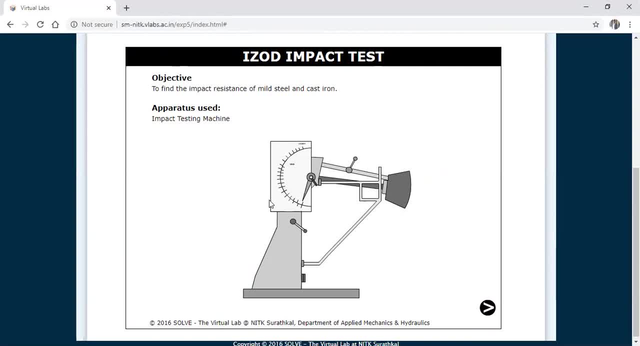 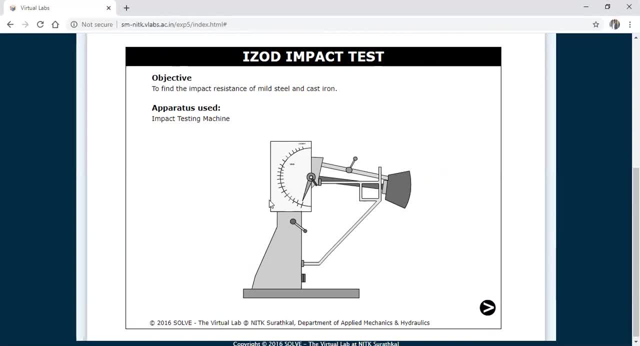 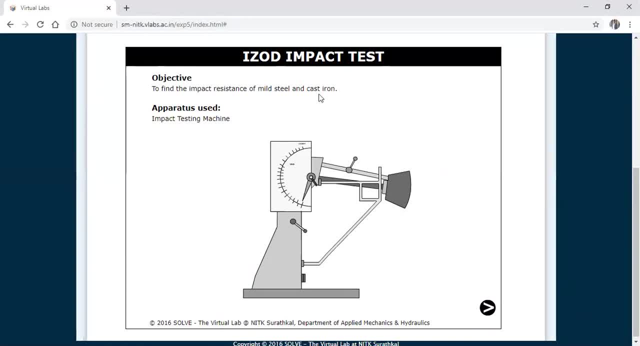 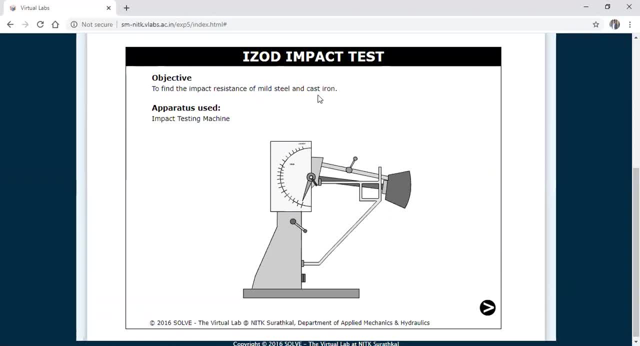 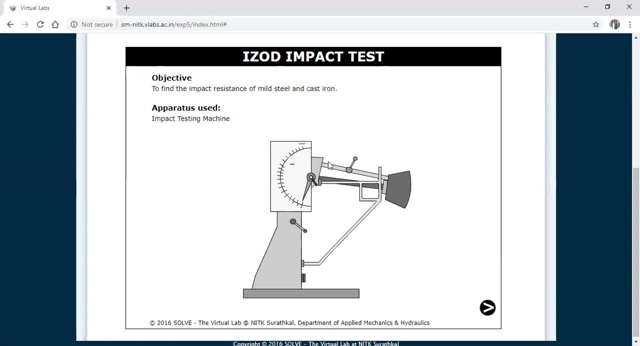 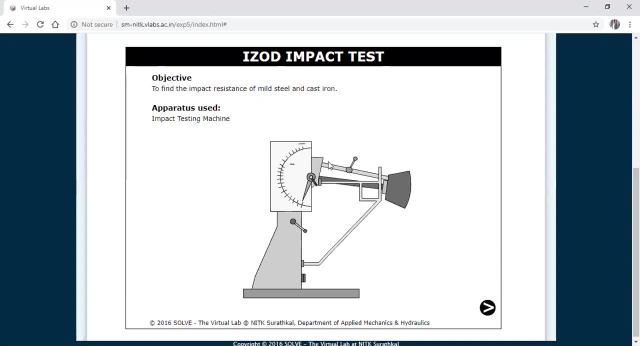 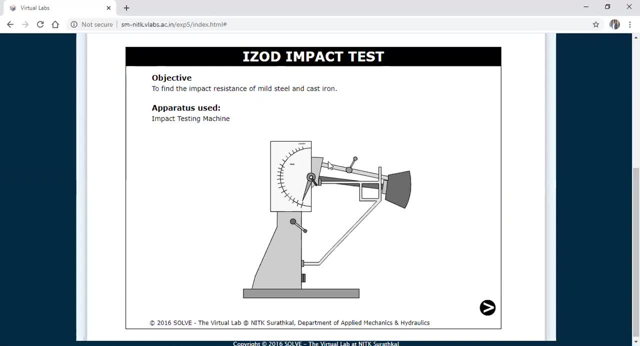 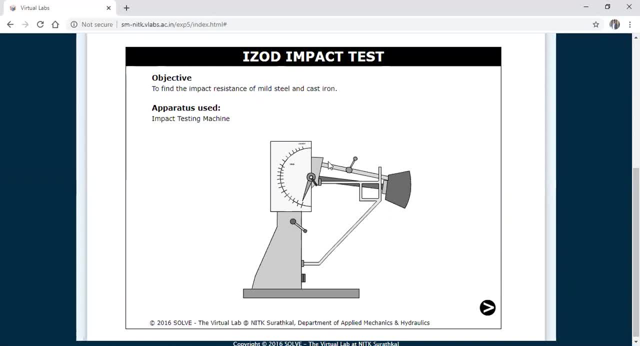 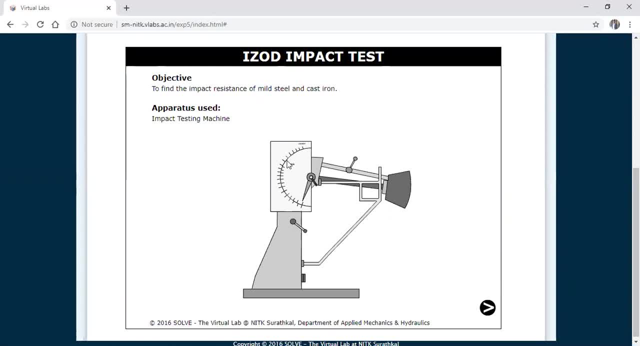 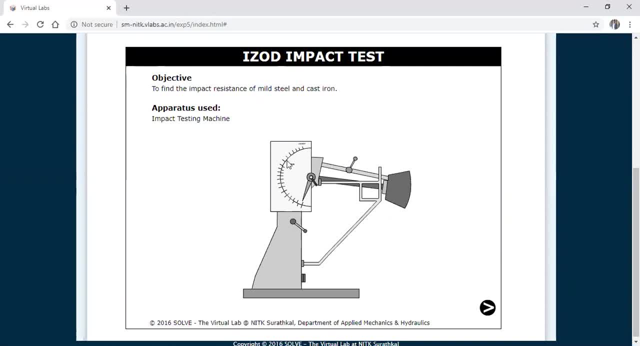 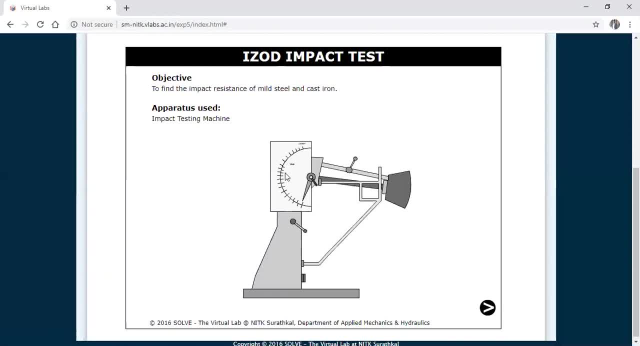 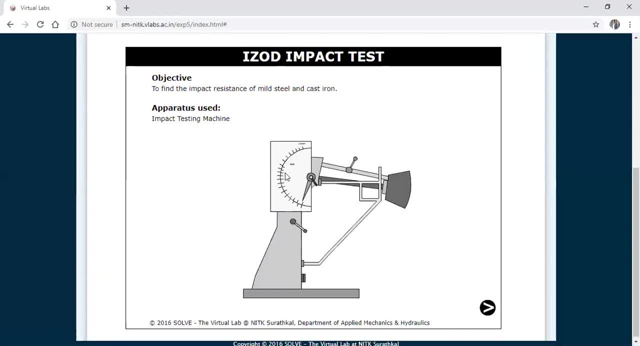 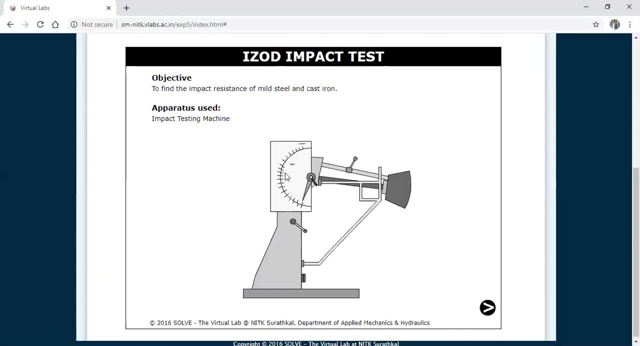 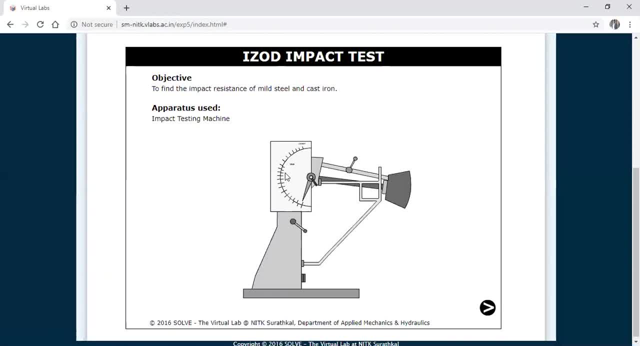 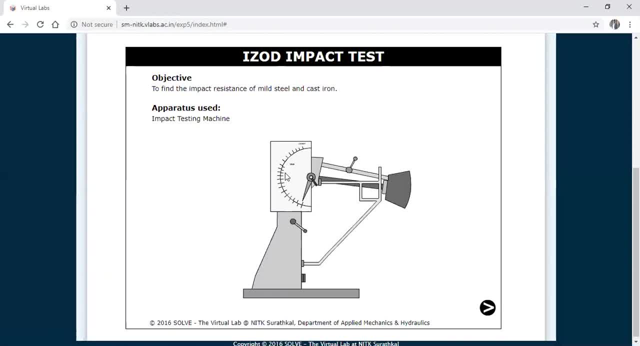 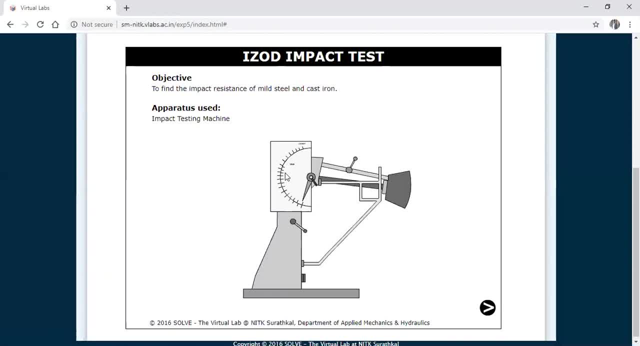 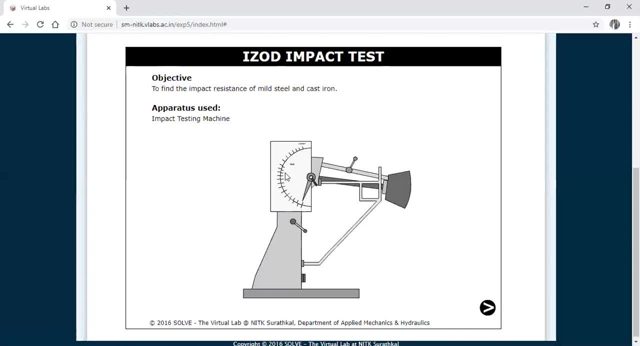 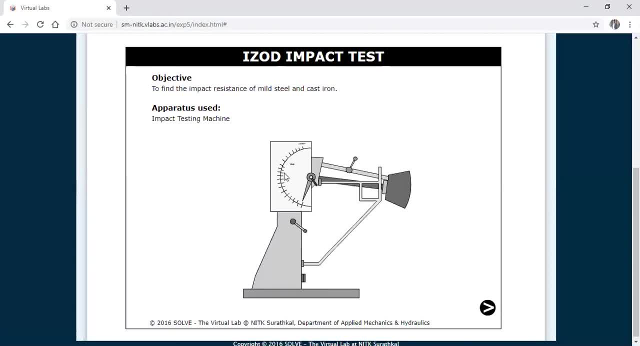 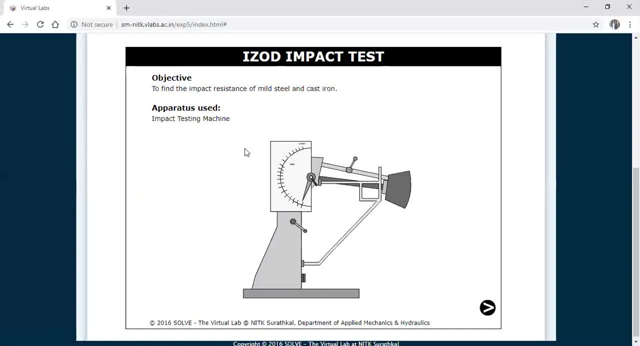 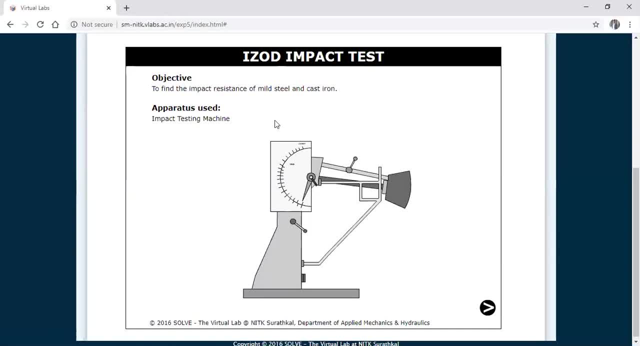 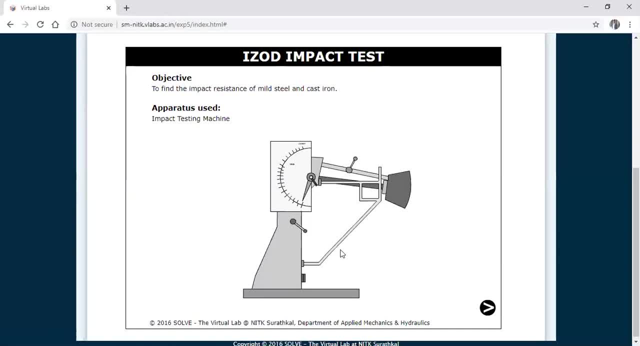 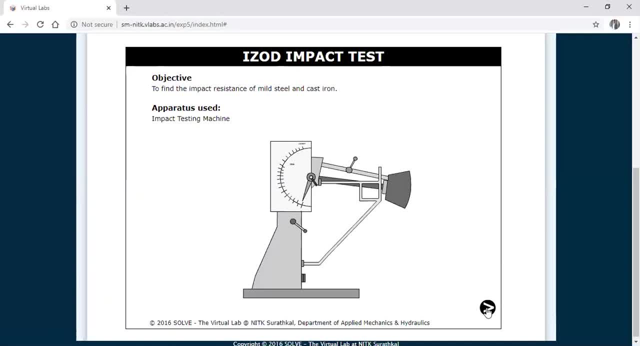 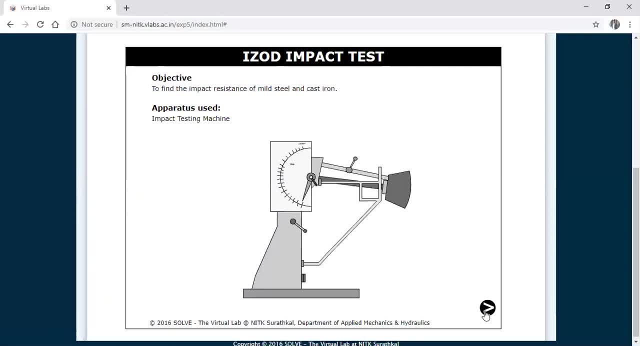 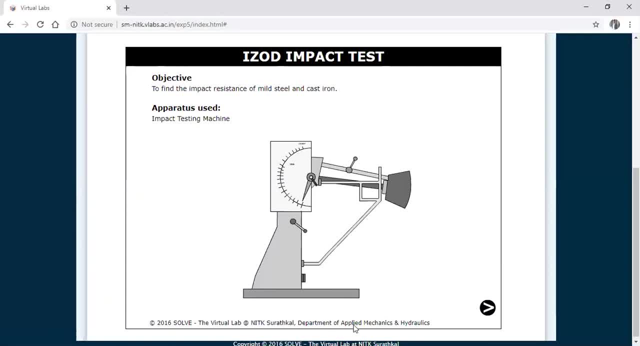 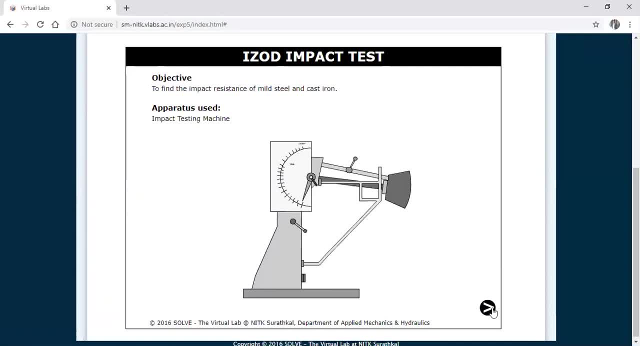 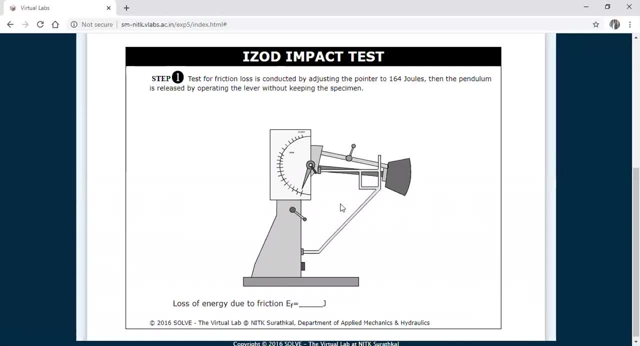 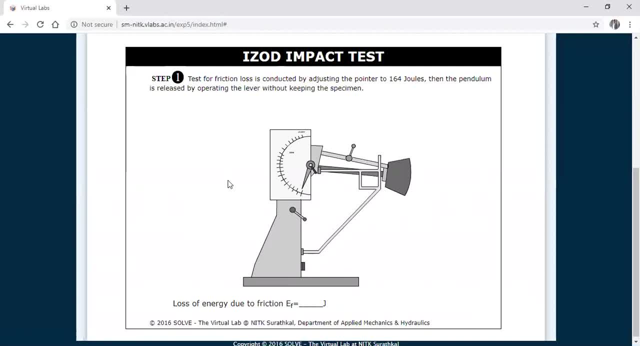 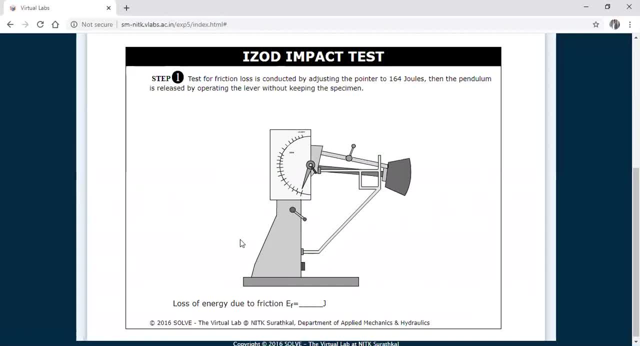 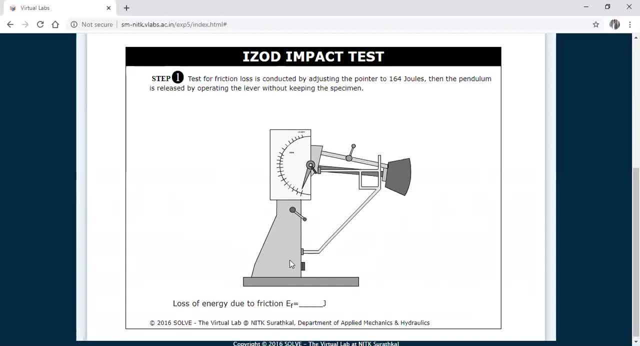 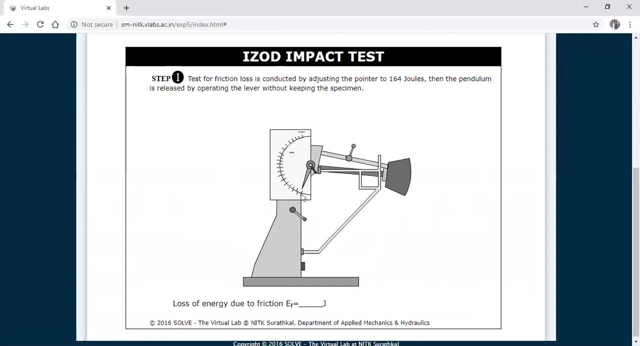 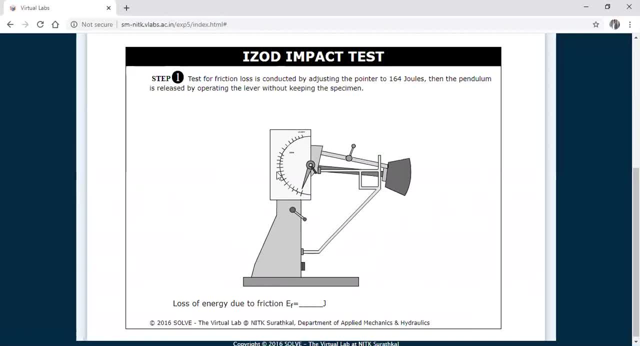 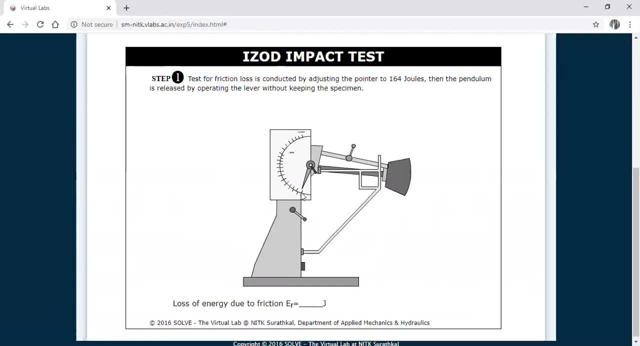 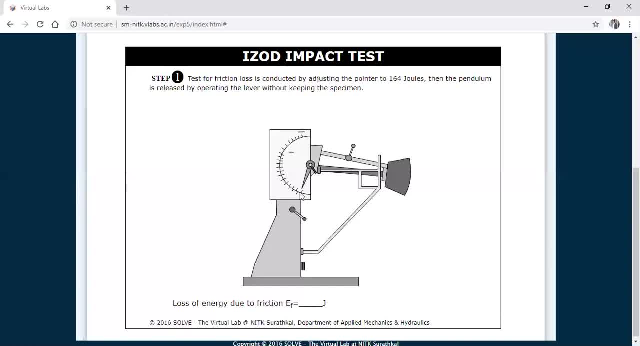 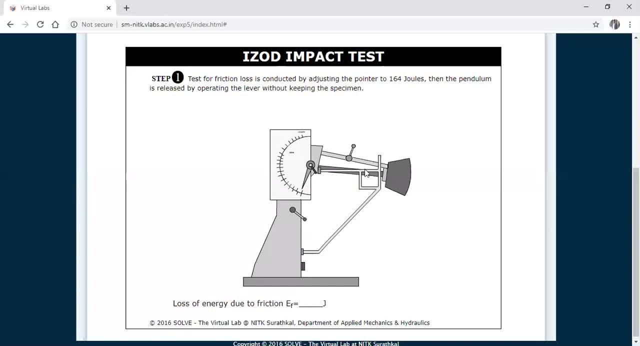 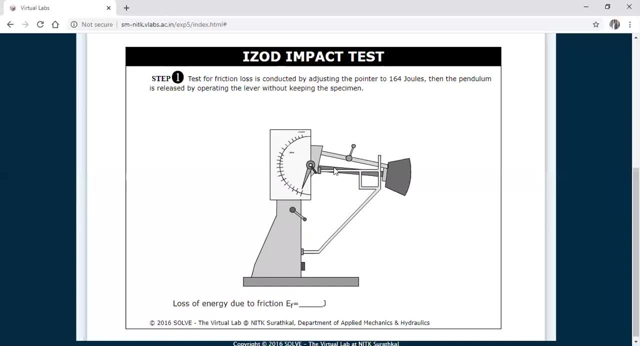 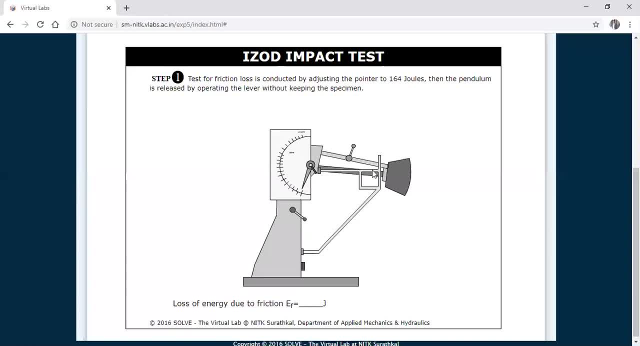 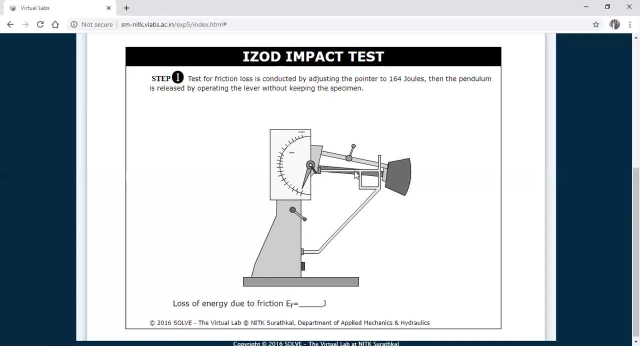 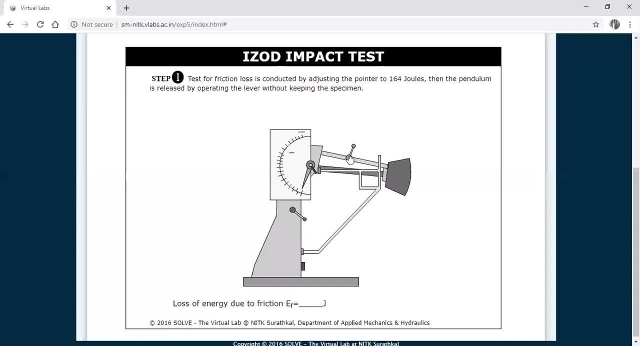 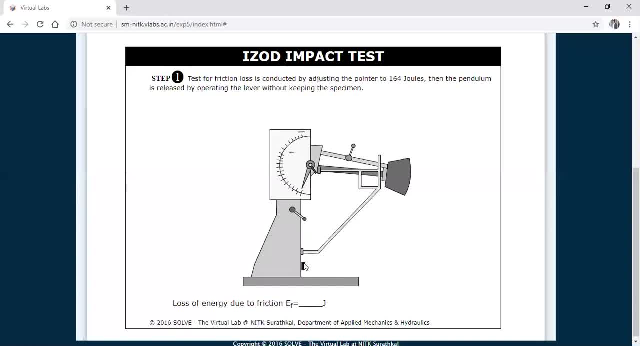 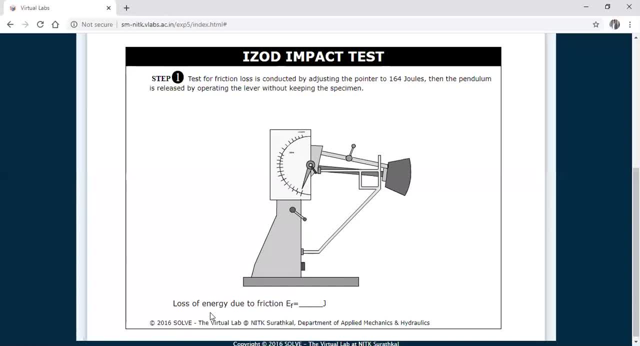 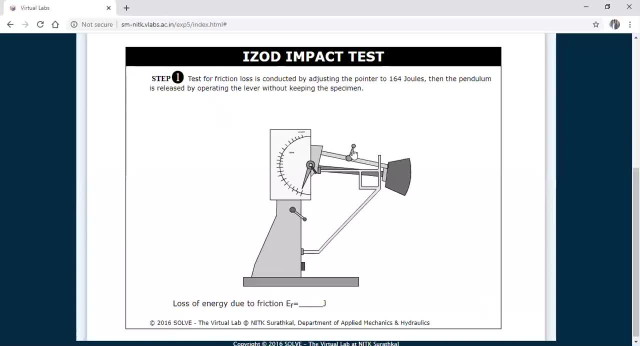 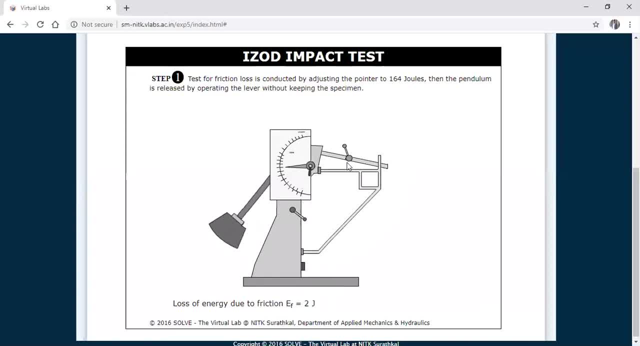 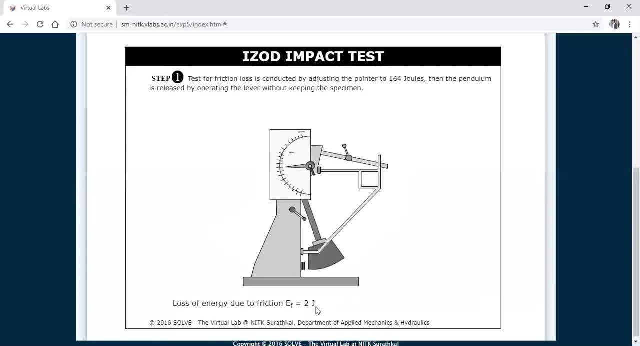 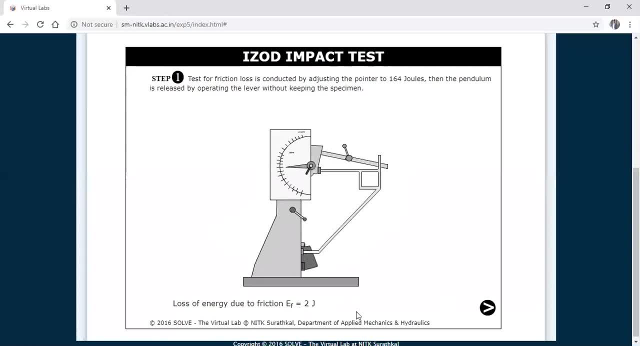 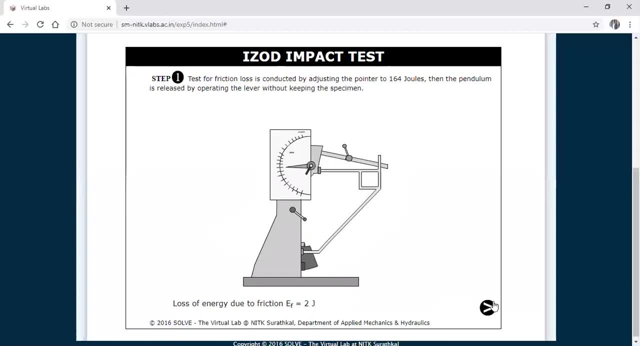 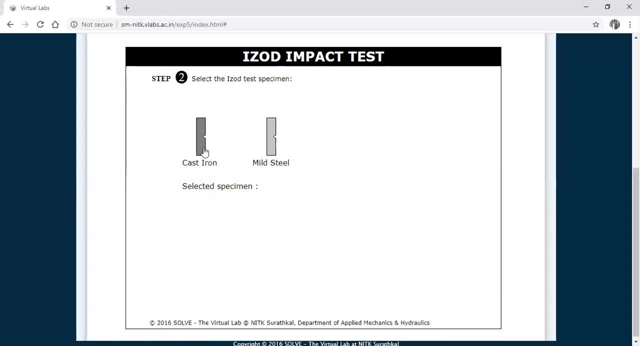 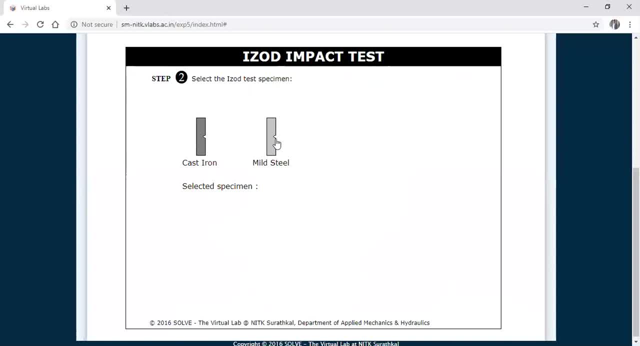 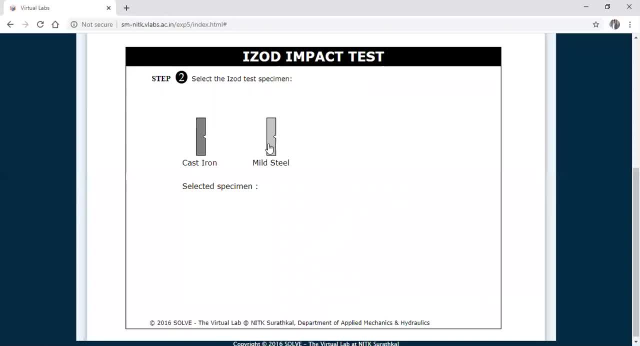 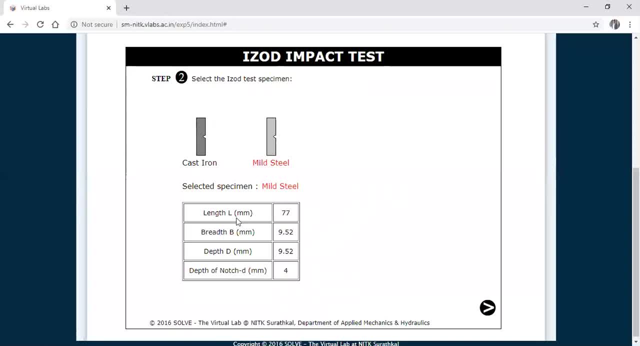 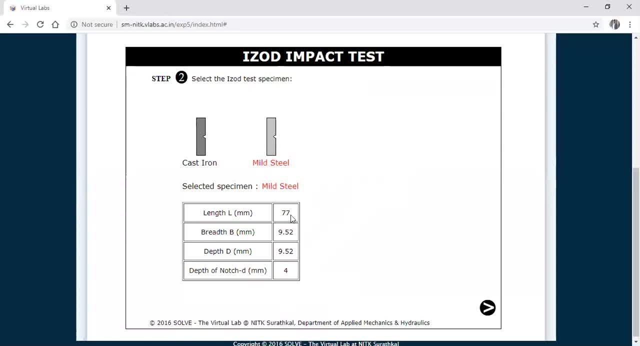 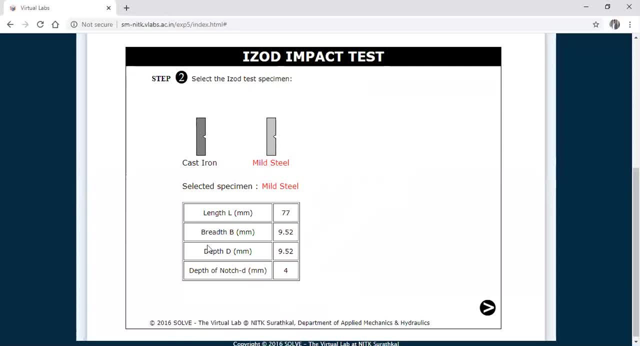 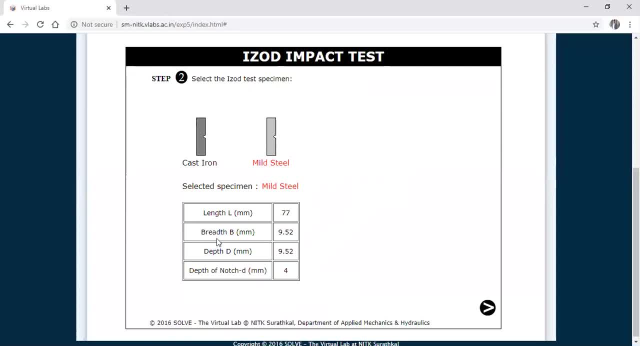 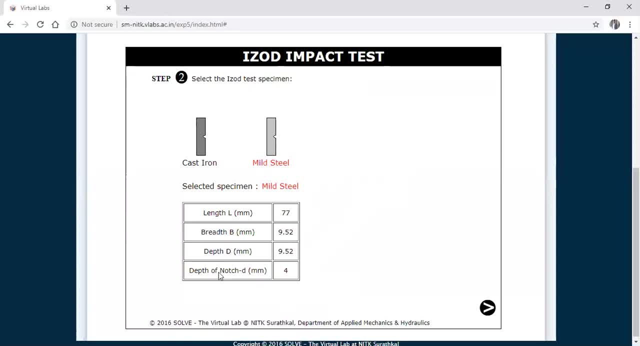 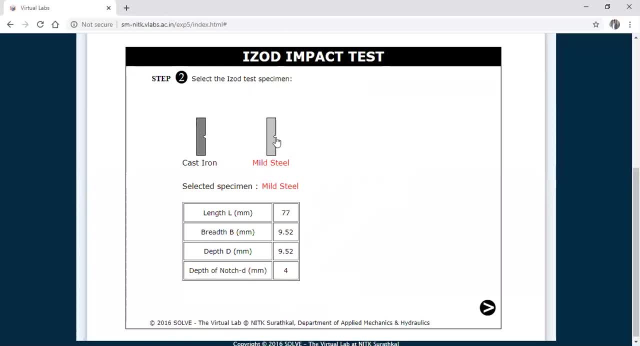 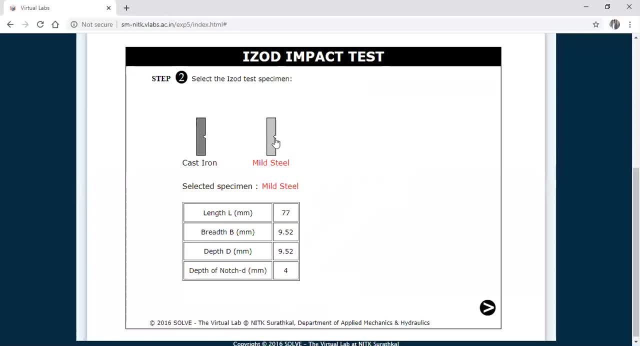 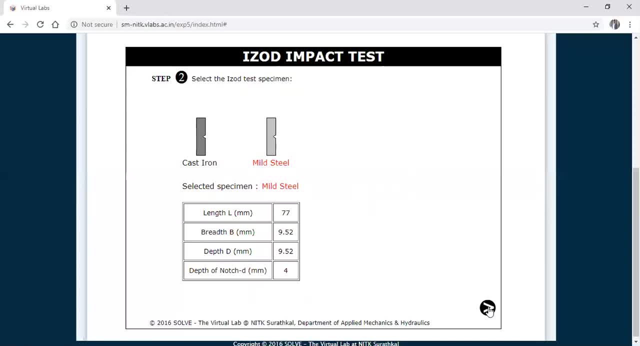 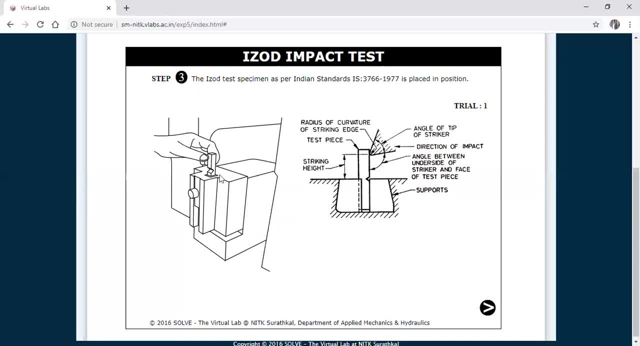 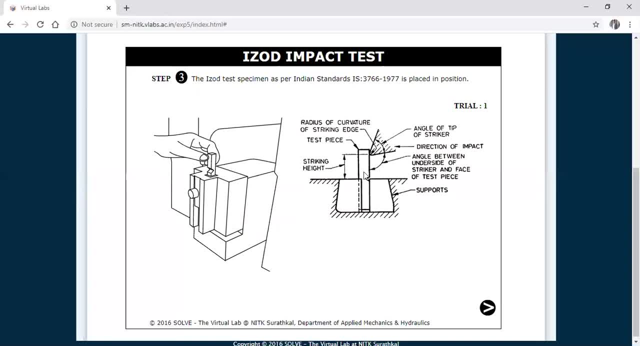 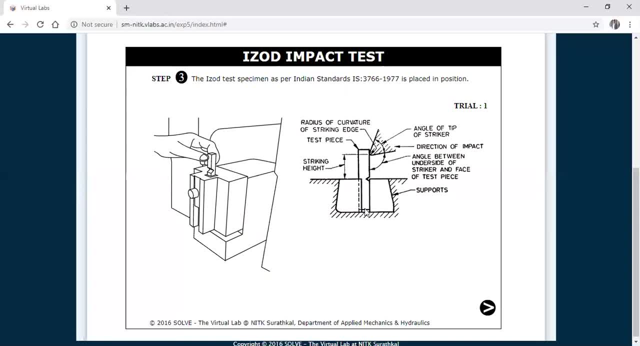 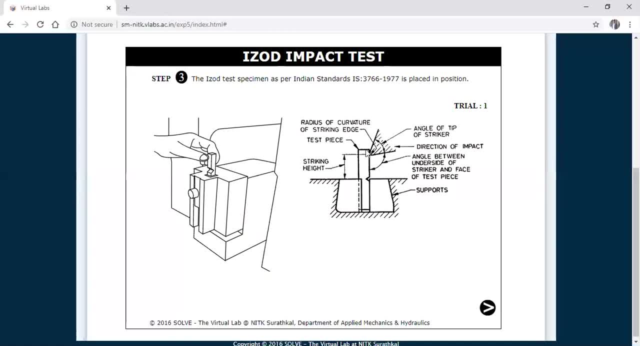 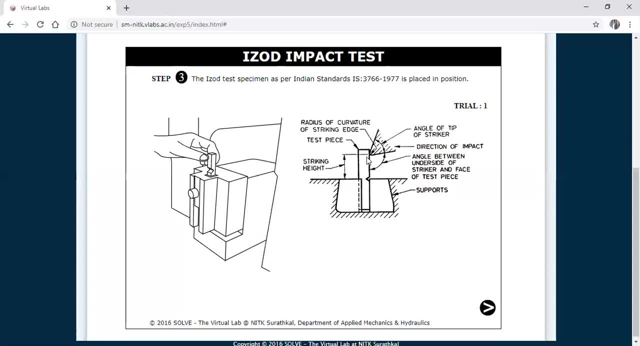 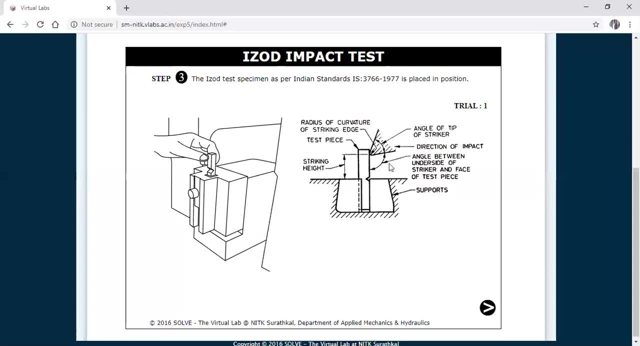 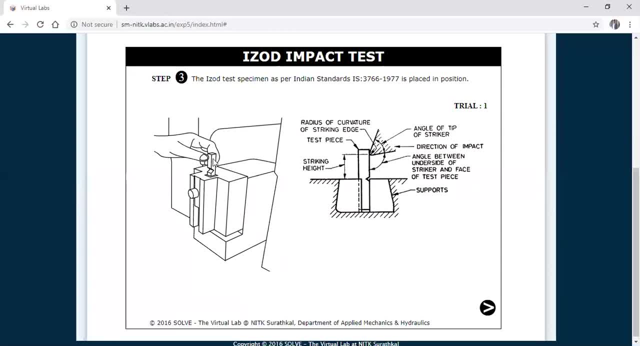 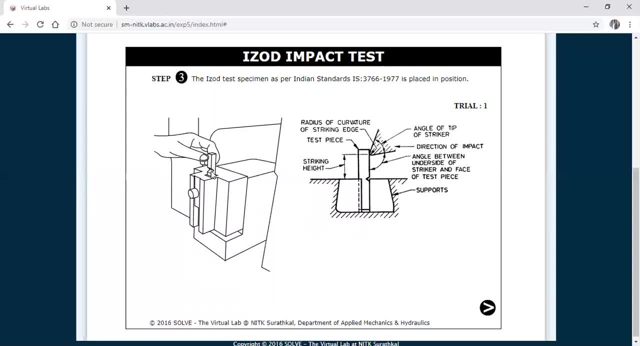 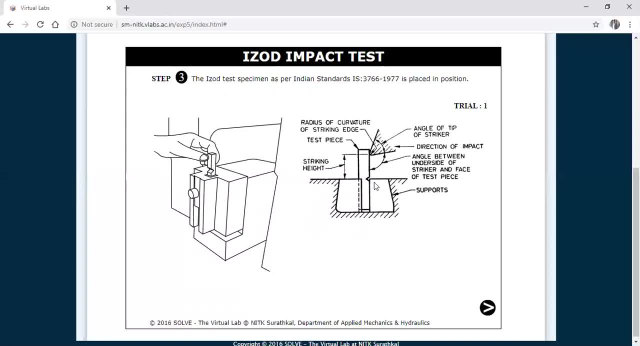 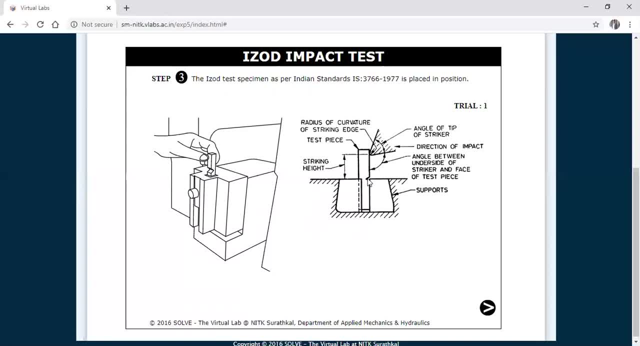 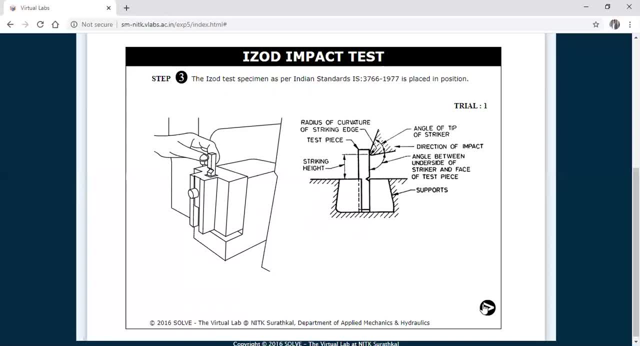 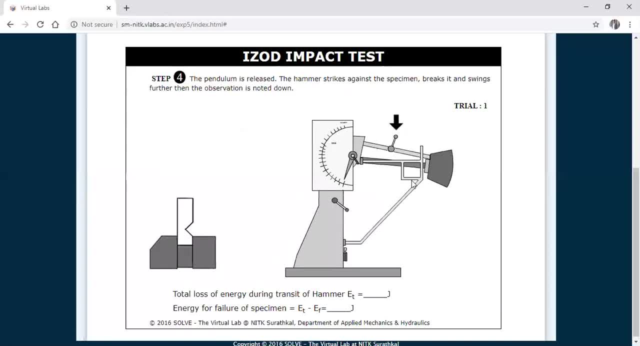 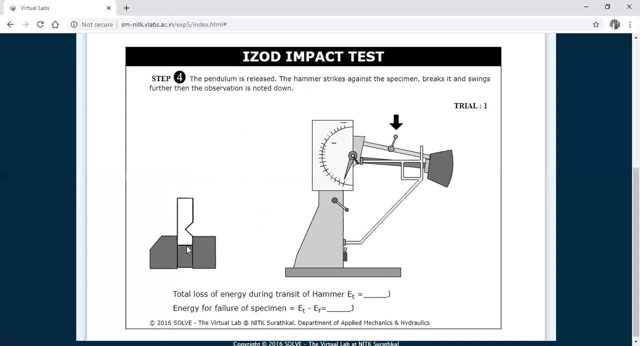 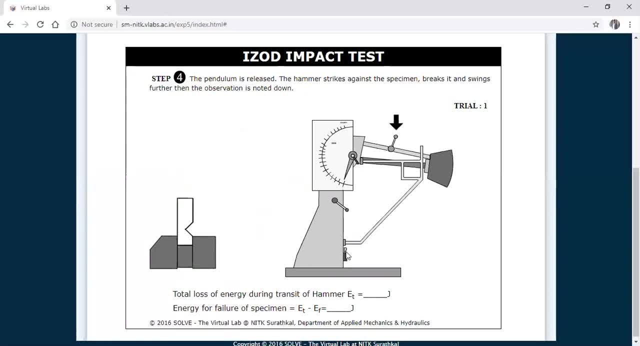 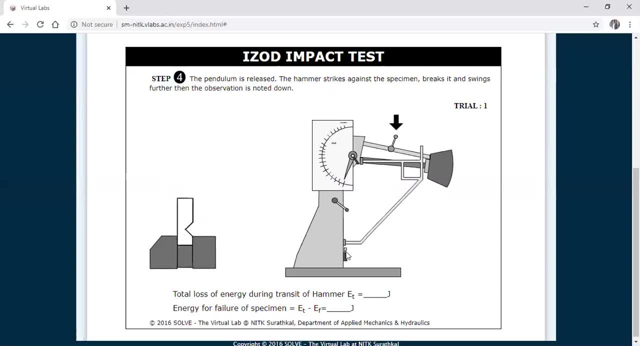 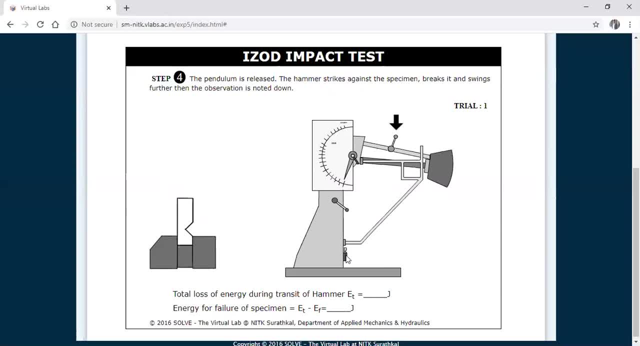 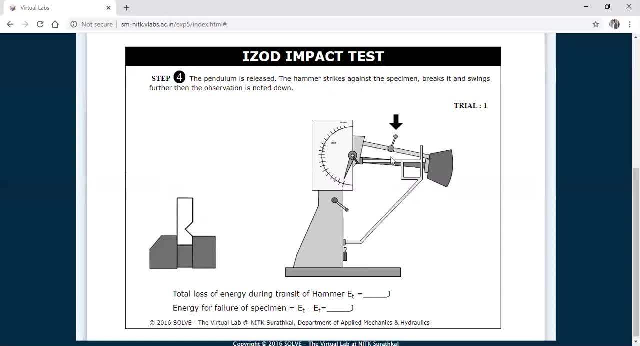 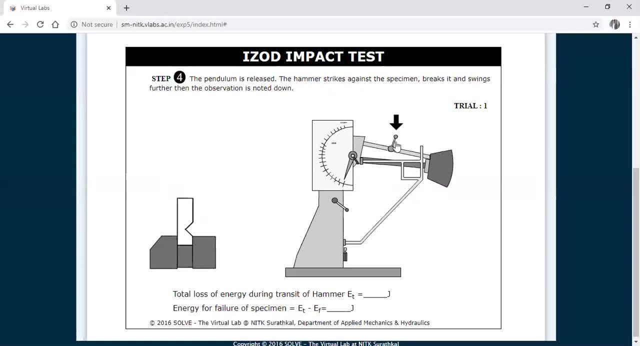 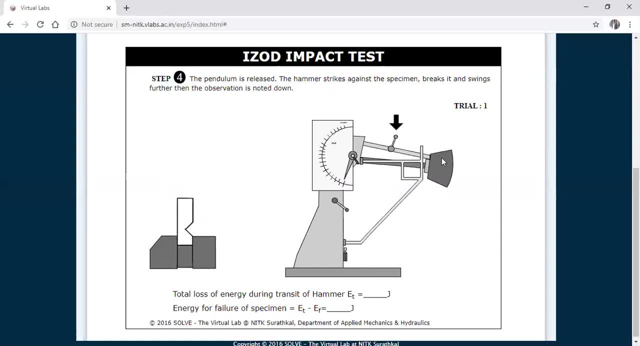 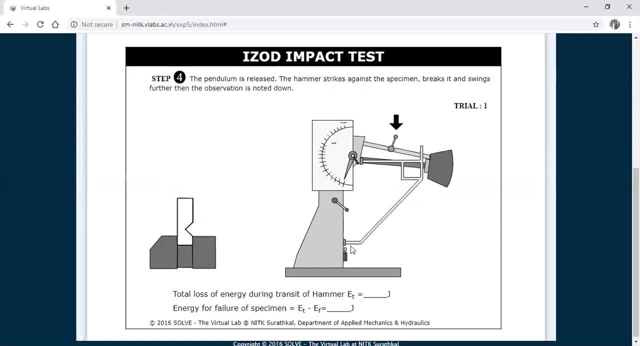 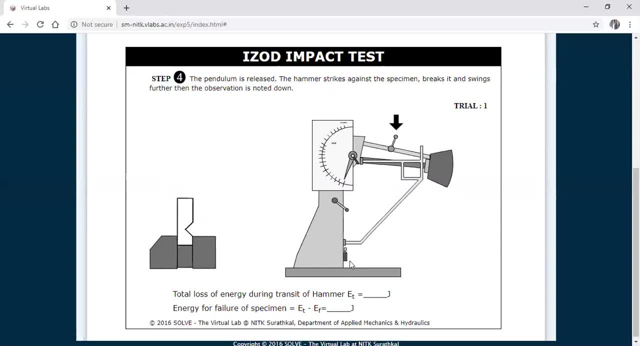 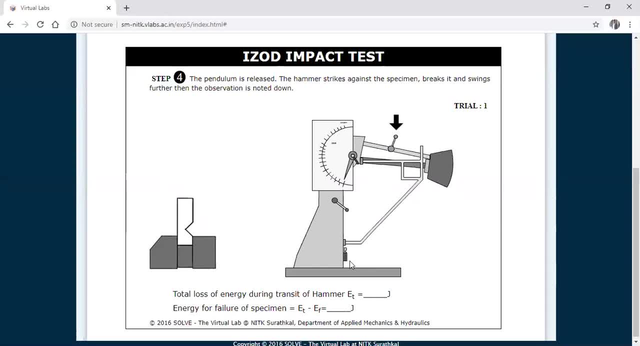 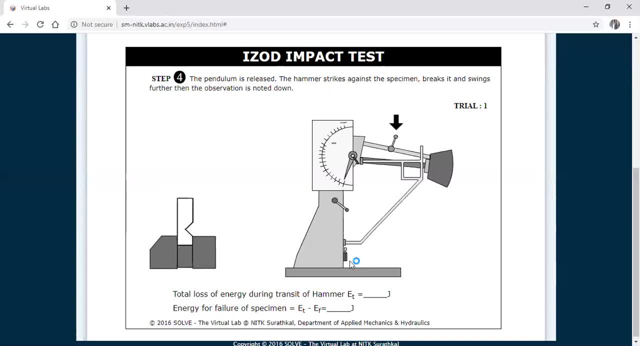 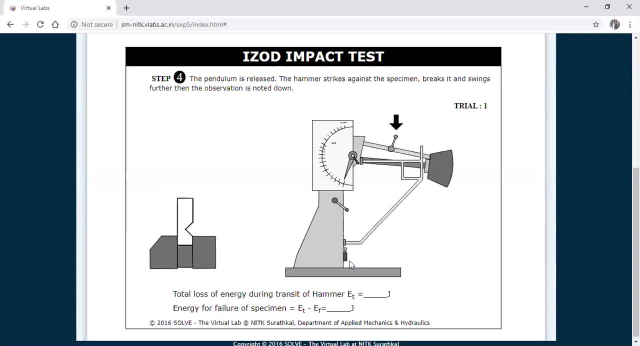 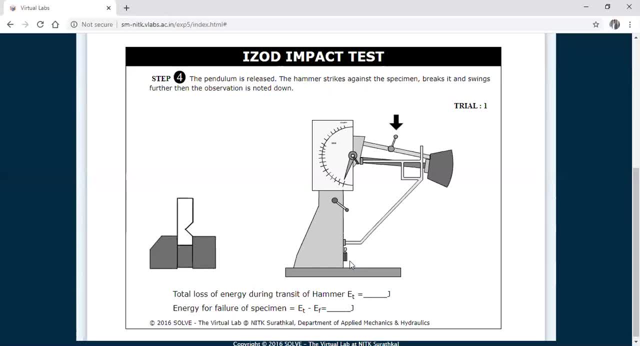 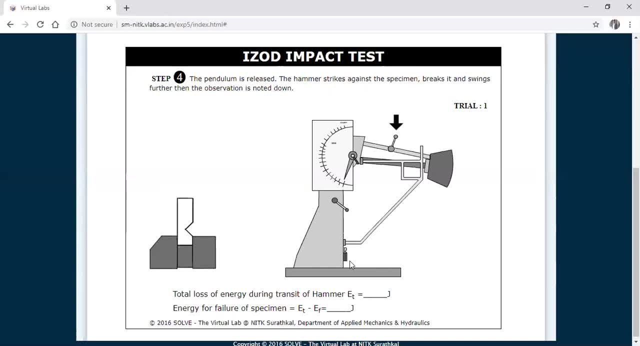 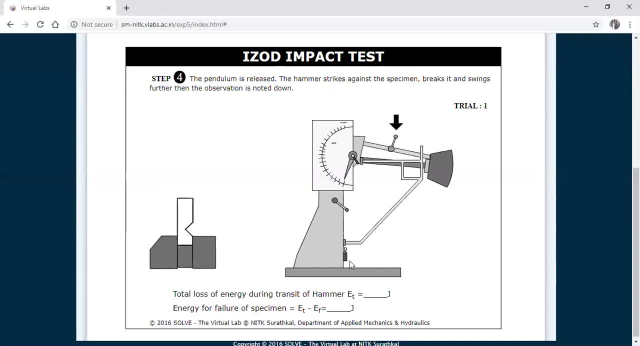 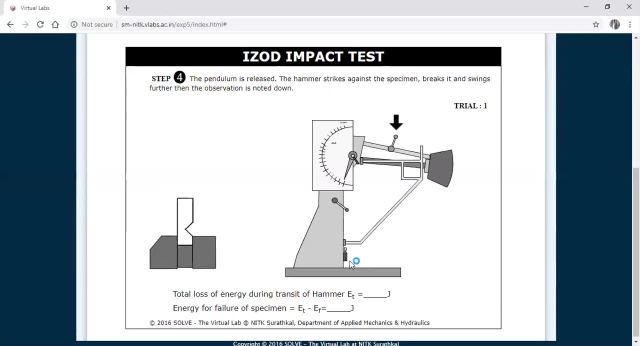 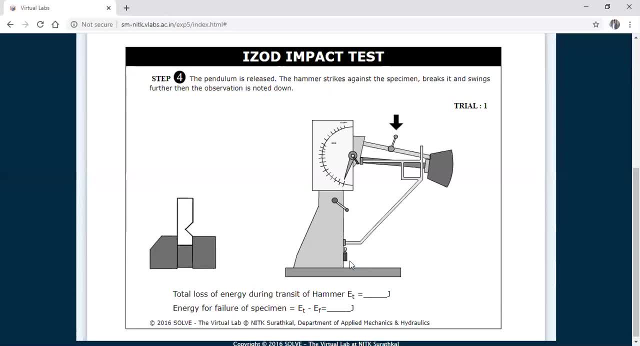 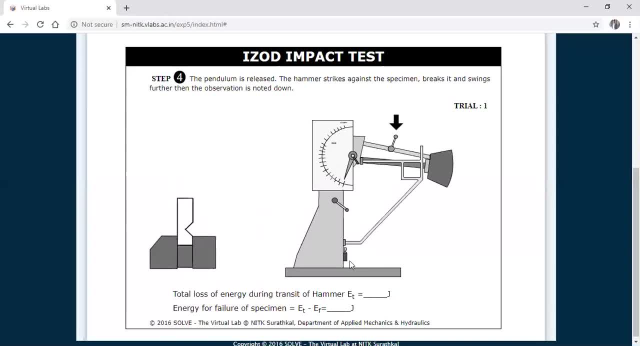 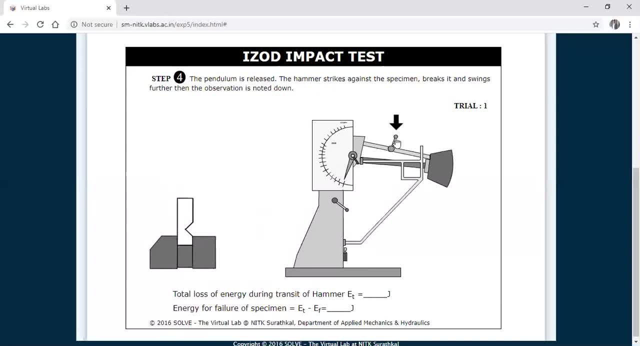 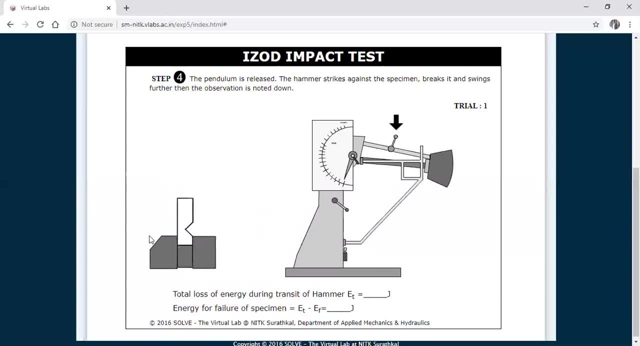 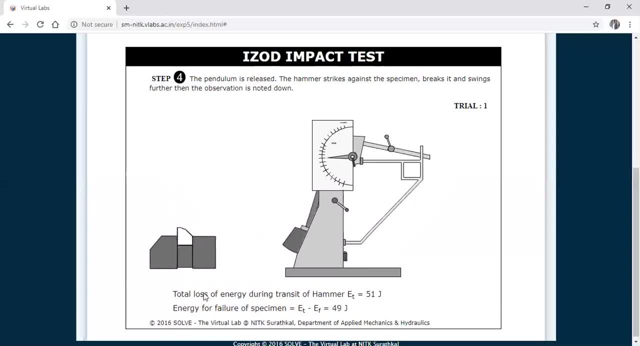 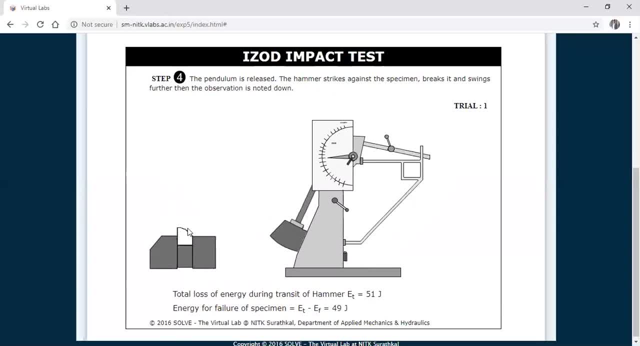 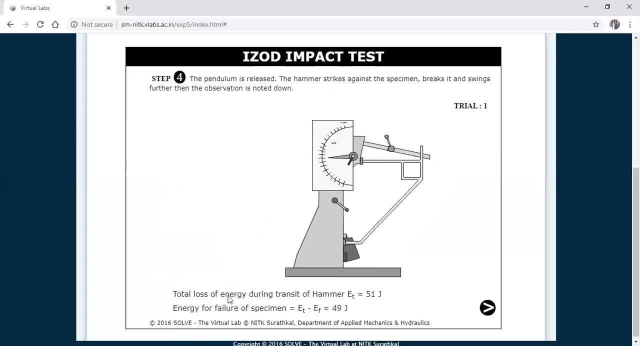 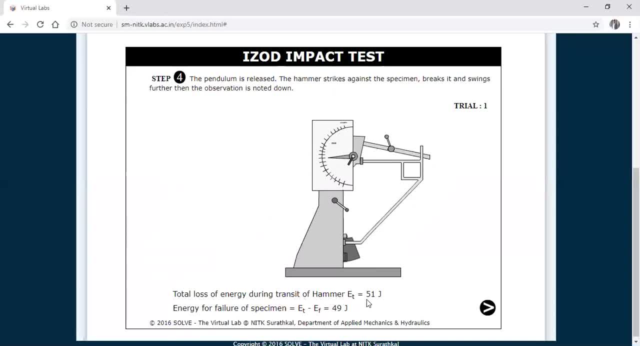 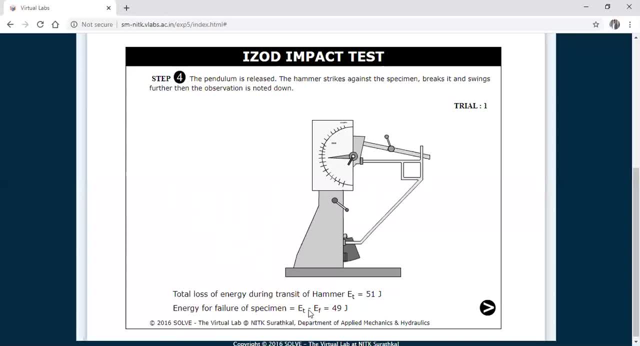 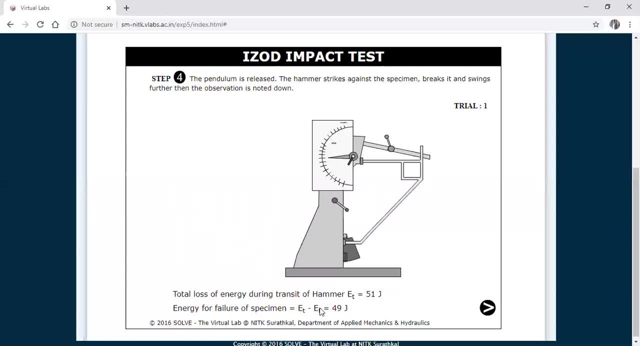 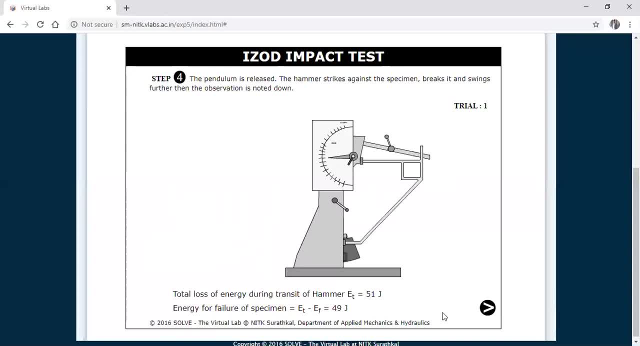 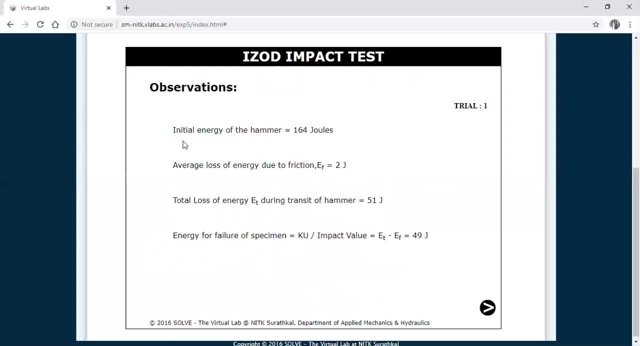 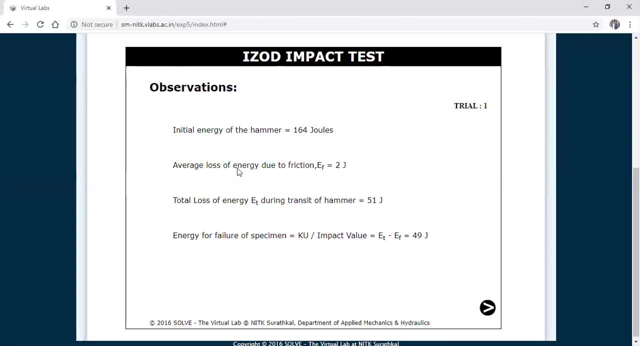 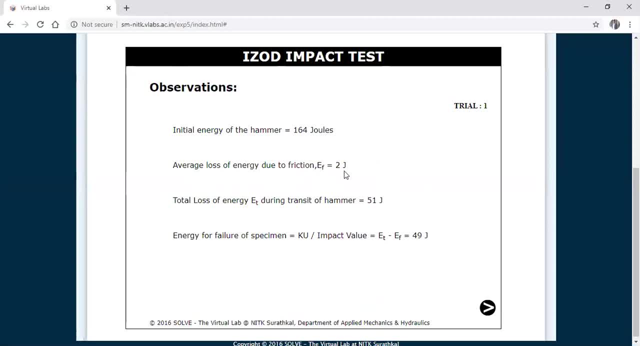 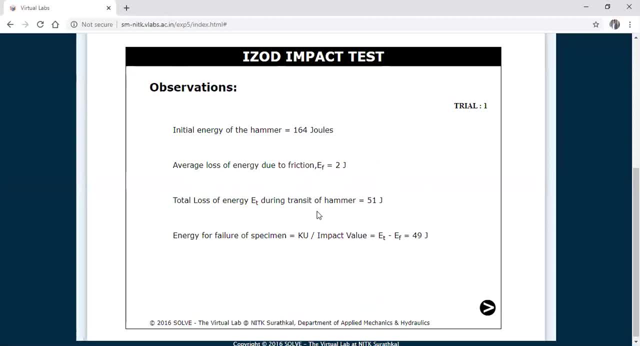 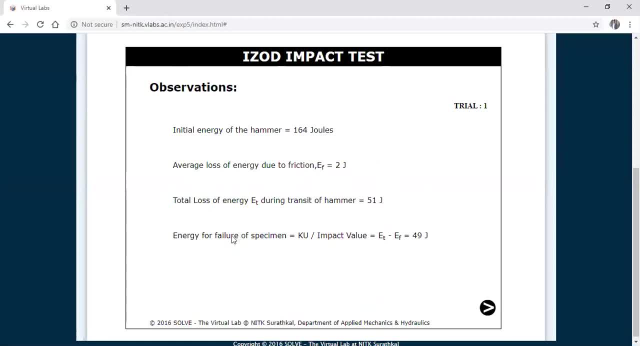 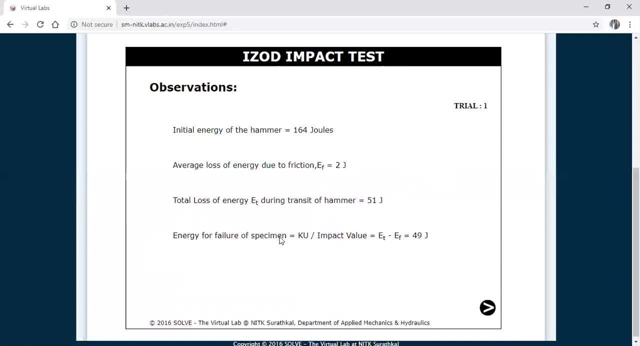 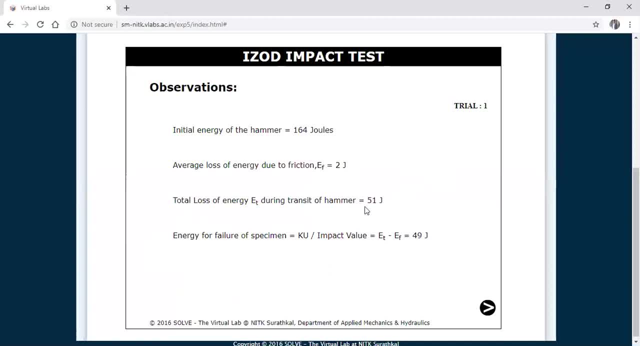 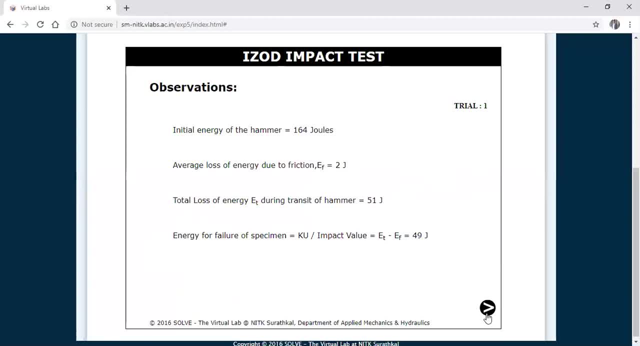 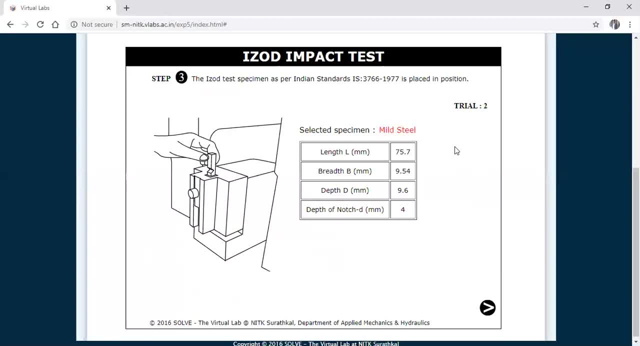 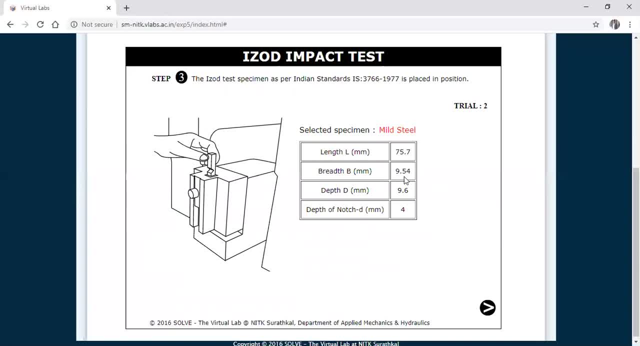 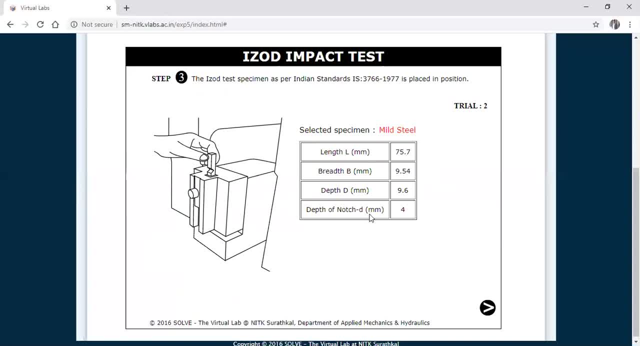 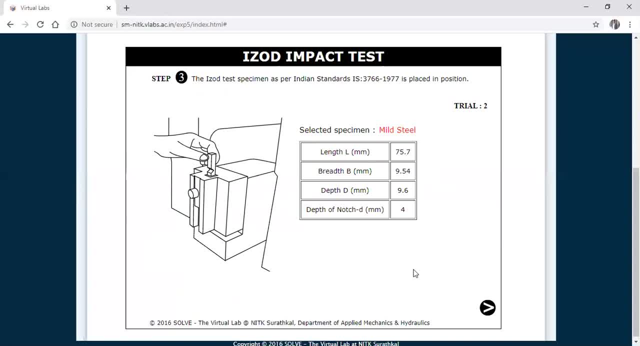 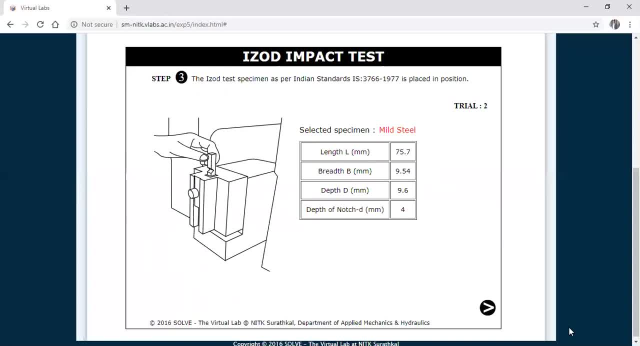 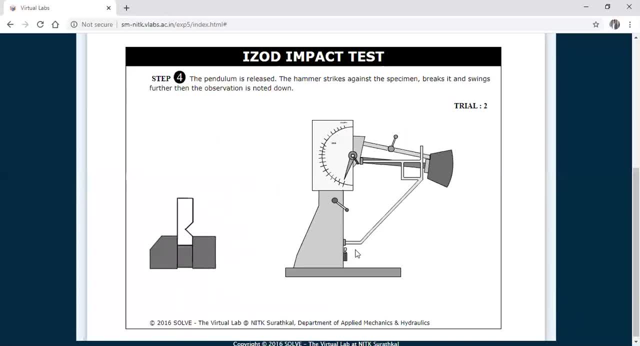 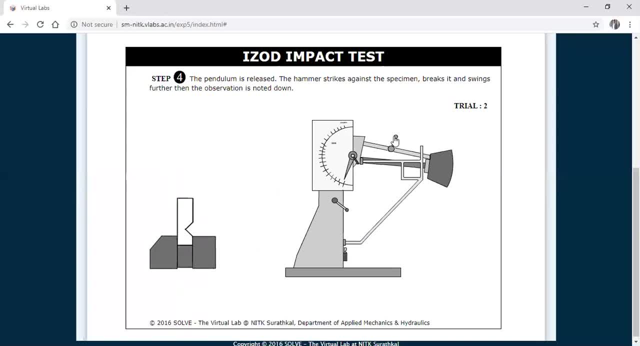 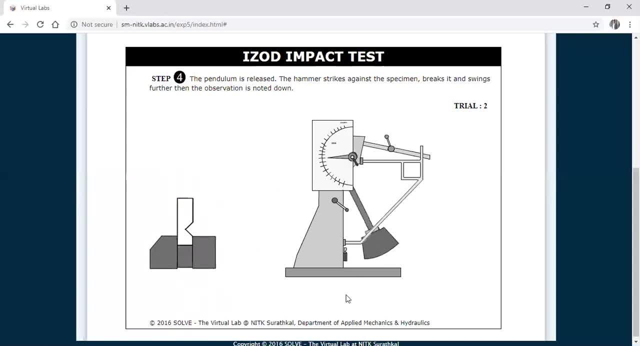 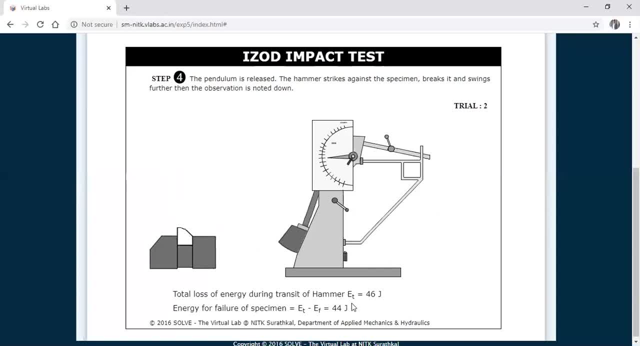 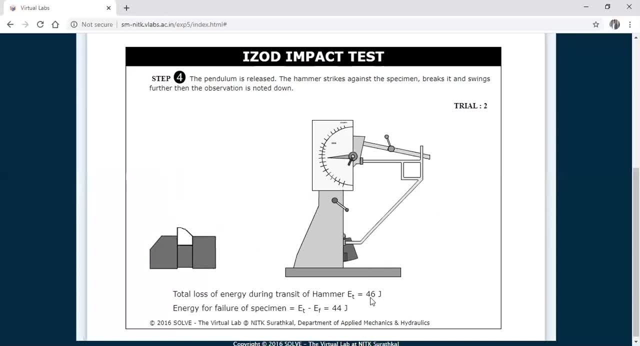 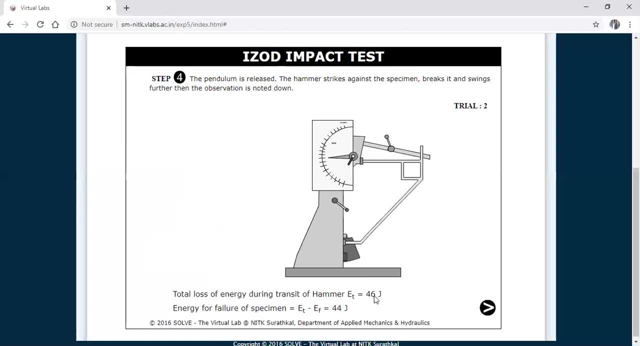 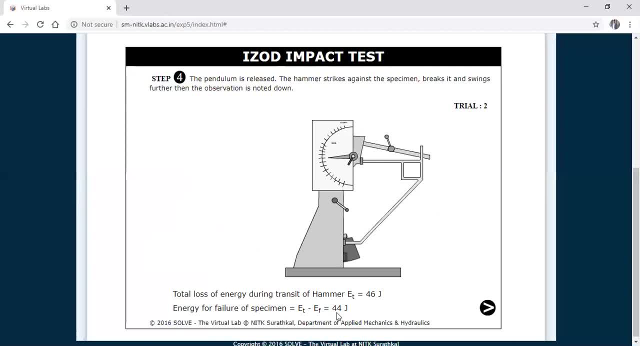 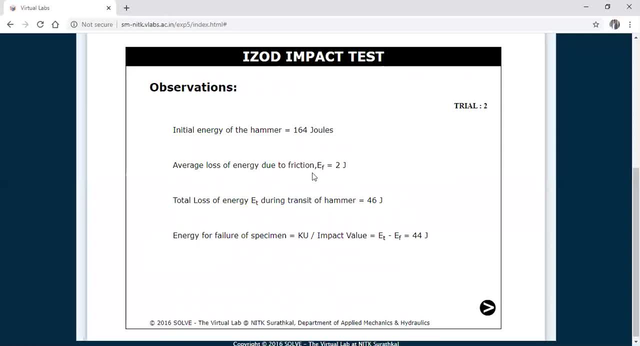 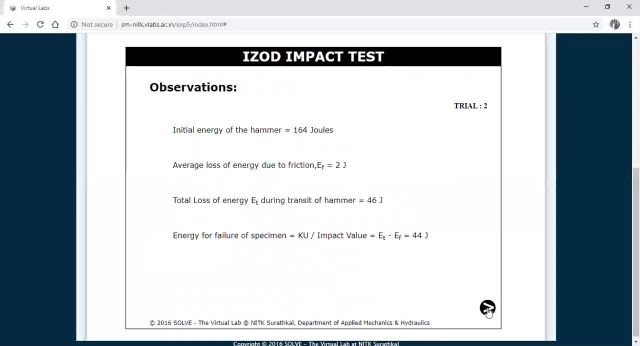 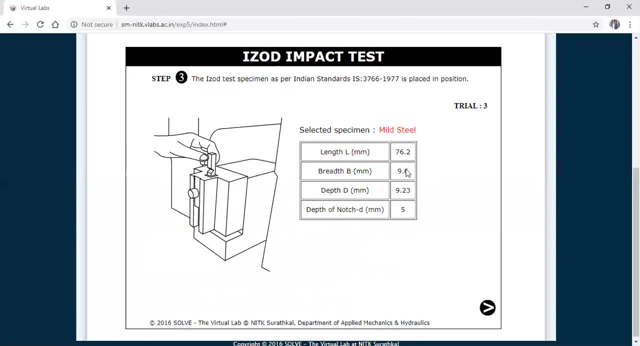 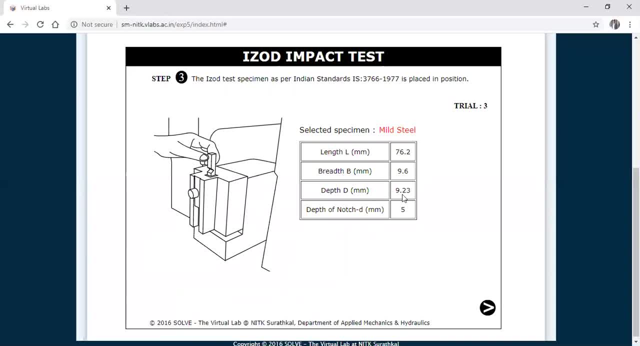 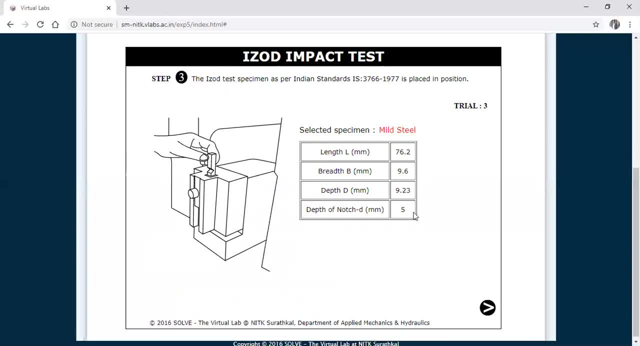 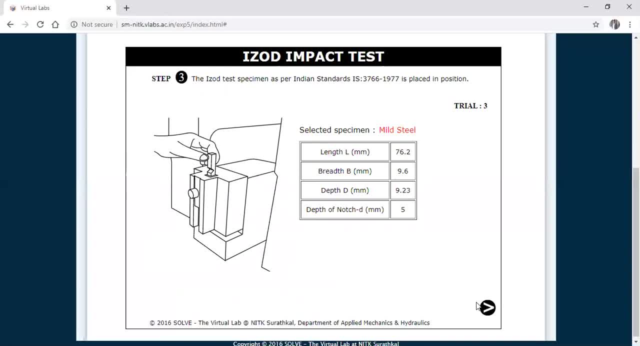 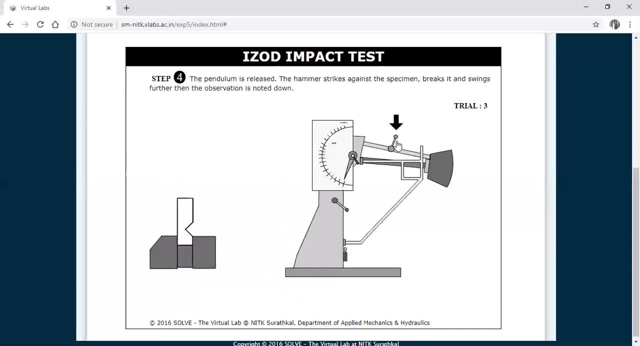 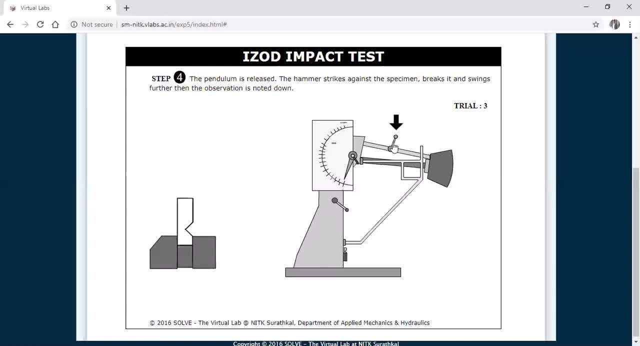 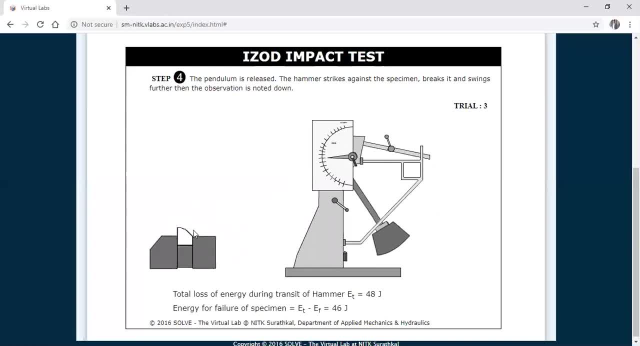 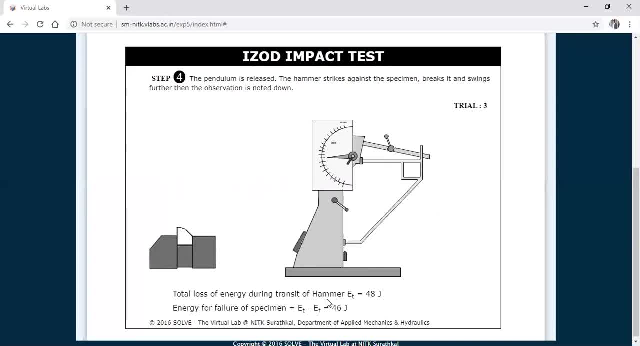 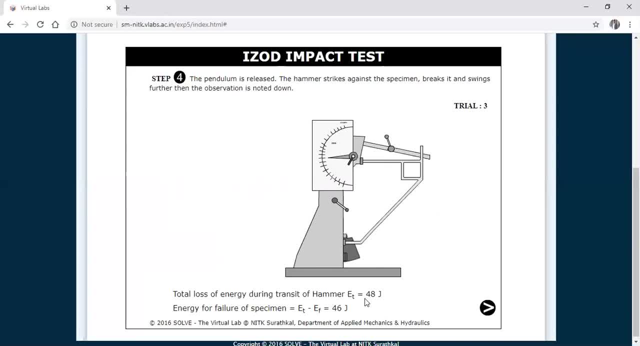 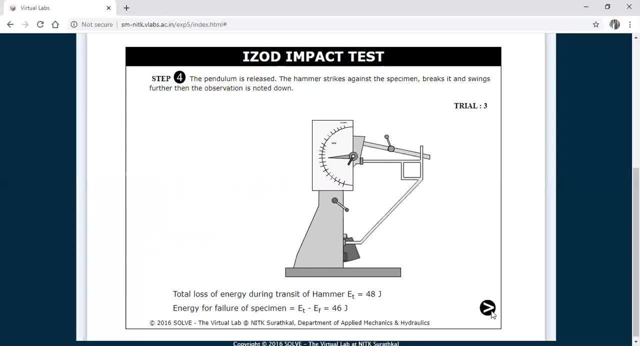 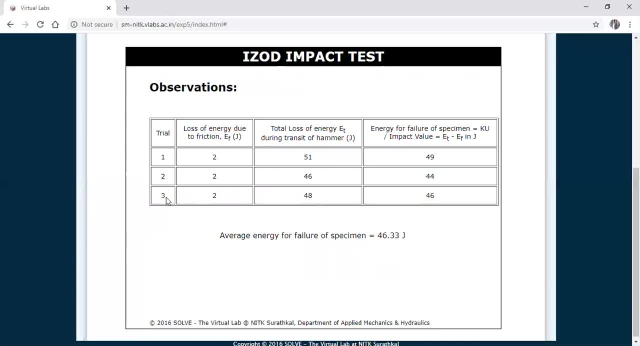 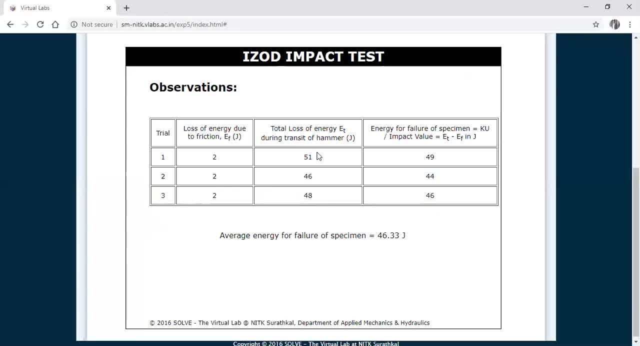 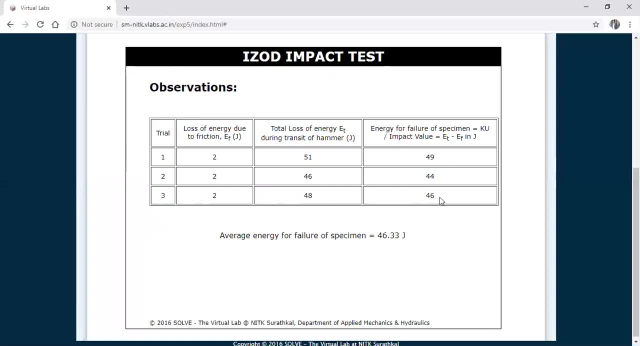 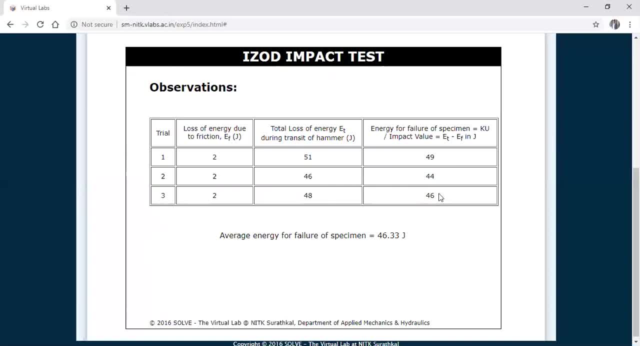 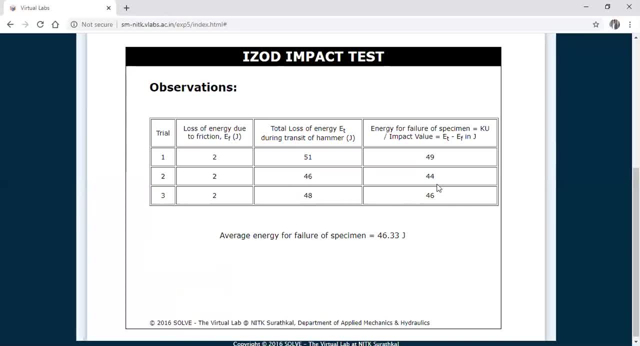